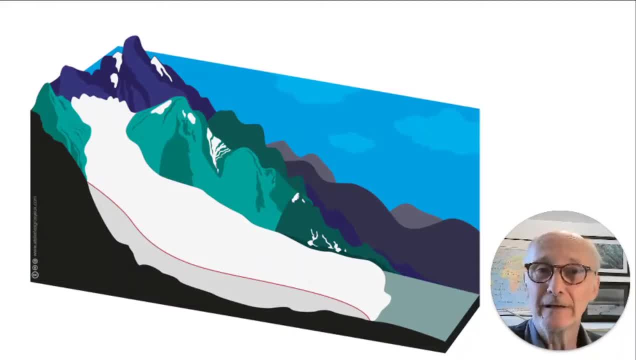 how you can translate them very easily. and they apply equally well to an ice sheet situation. And we're dealing in all of this with surface mass balance. There's also a mass balance to worry about in the interior and the base of the glacier, but we're just talking about 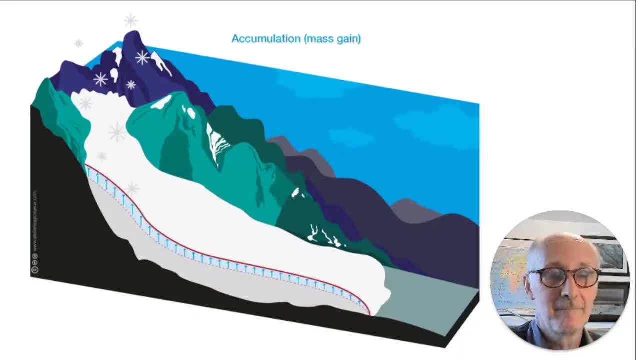 surface mass balance of glaciers. Mass balance is all about the balance, or the budget, between inputs and outputs to and from a system. In a glacier system, the input is the input of precipitation or snow in the form of accumulation. In this diagram, over the course of time, a layer of snow is building up on the glacier. You can 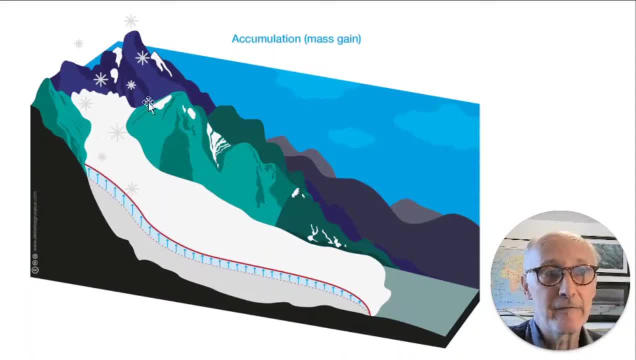 see they've drawn it here where a little bit more snow is building up in the higher layers of the glacier, in the higher altitudes, the colder environment, the snowier environment and a little bit less down at lower elevations. That might vary from glacier to glacier. 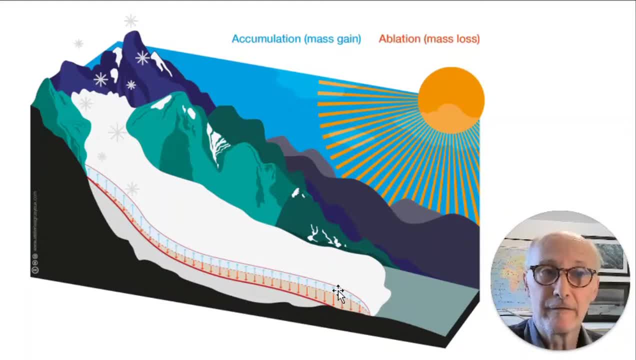 Also through the course of the year there is mass loss from the glacier: ablation, melting of the snow and ice carving of material off the front of the glacier. We'll look at that in another part of the session. But there's both accumulation gain of mass and ablation loss of mass. 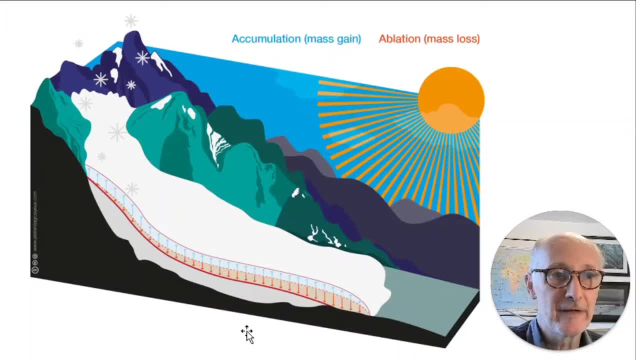 over the course of the year And they've superimposed the two on the diagram here And if you sum those two effects together then we have this overall picture. So if you add the accumulation and take away the mass loss over the course of the year, that's giving us 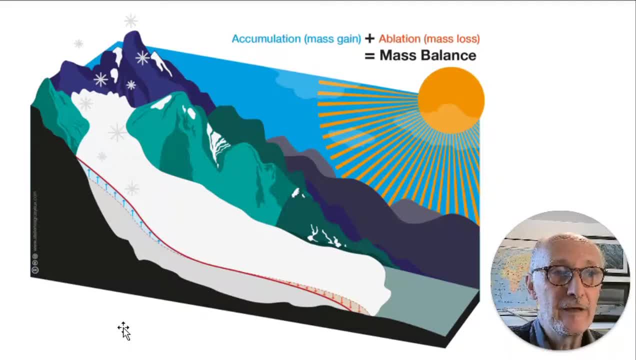 an annual mass balance And over the course of the year. here you can see that there's more accumulation than there is ablation in this upper area of the glacier, But there's more ablation than there is accumulation in the lower area of the glacier. So overall we have a mass. 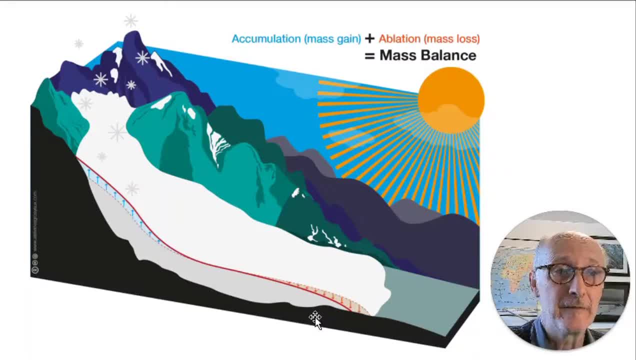 loss or a negative balance, a negative mass balance in the bottom of the glacier and an overall mass gain or a positive mass balance at the top of the glacier. In a glacier that is in some kind of equilibrium, that difference will be balanced by movement of ice from the upper areas of the glacier through the glacier. 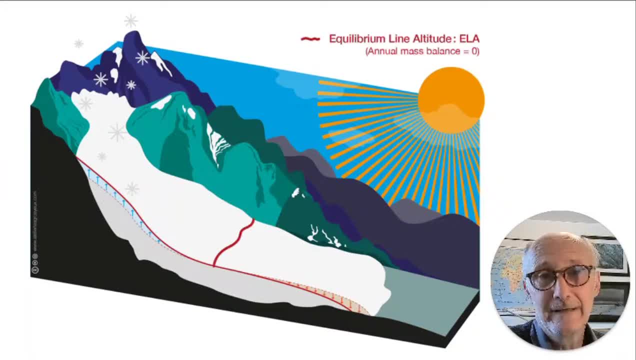 to the lower areas of the glacier. In between the upper area of accumulation and the lower area of ablation, the accumulation area and the ablation area, there's a zone or a line across the glacier where, locally, the mass balance is zero. The amount of 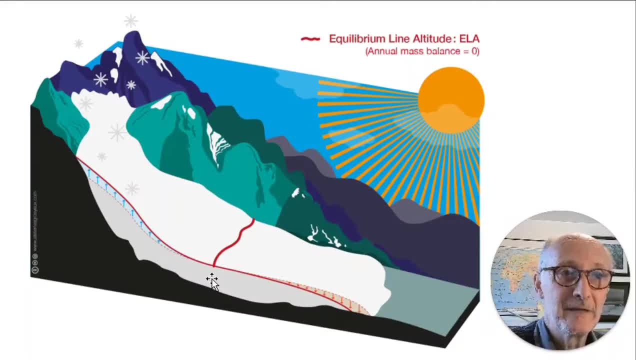 accumulation is equal to the amount of ablation. That's referred to as the equilibrium line, and the position of the glacier where that line occurs is referred to as the equilibrium line, altitude, the ELA- and that's a very important concept in glaciers when we're thinking about how glaciers advance. 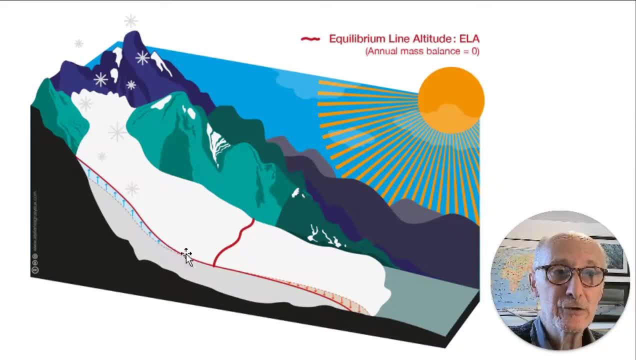 and retreat in response to climate change, because changes in the position of that equilibrium line change the accumulation area ratio, In other words the ratio between the size of the accumulation area where the glacier is being fed and the size of the ablation area where the glacier is losing. 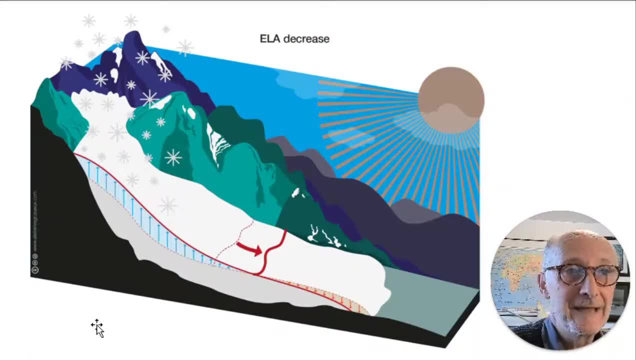 material. So if the ELA decreases, the altitude of the equilibrium line decreases, then the accumulation area increases. So we're getting overall equilibrium, A greater amount of input in the accumulation area and the ablation area where we're losing material, that shrinks In that situation. other things: 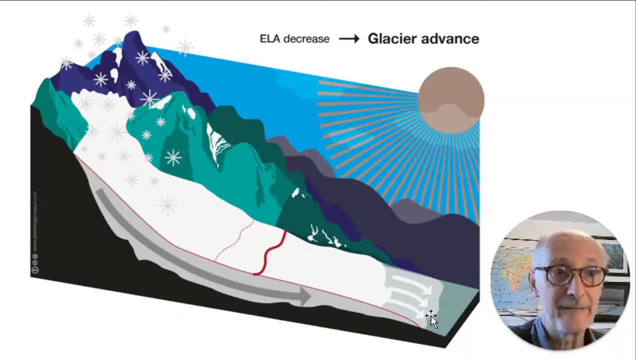 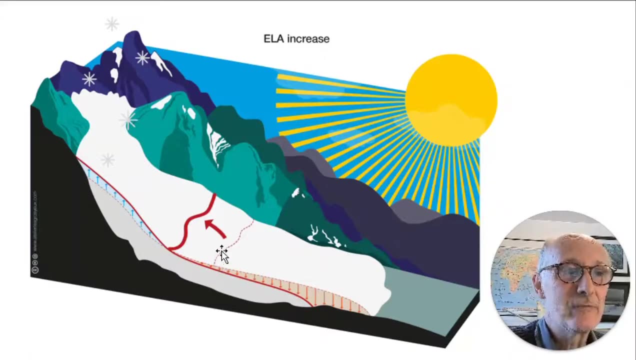 being equal, you might well expect the glacier to be healthy and expanding and advancing. So if the ELA is decreasing, is lowering, then we're likely to have a healthy, advancing glacier. By contrast, in warmer conditions, when there's more melting, less accumulation, the equilibrium 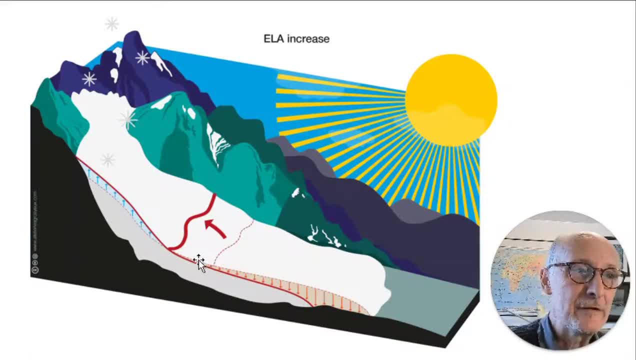 line is rising up, the altitude is increasing, the equilibrium line is moving up the glacier, then we're shrinking the accumulation area, we're expanding the ablation area and the consequence of that is likely to be retreat of the glacier. So there's a very straightforward correspondence there. 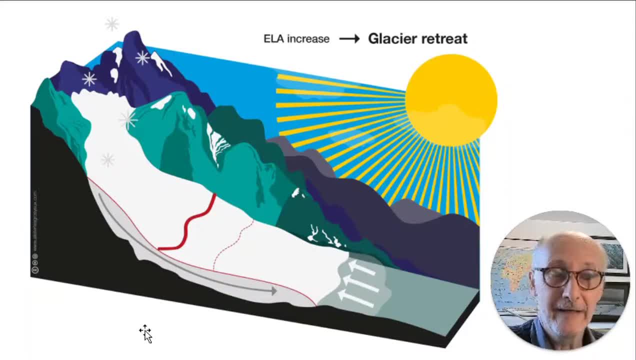 between inputs, outputs balance and the health or expansion and contraction of the glacier, And we're going to look at that in a little bit more detail in the later sections of this year. I just want to draw up those mass balance ideas that you've already seen in a 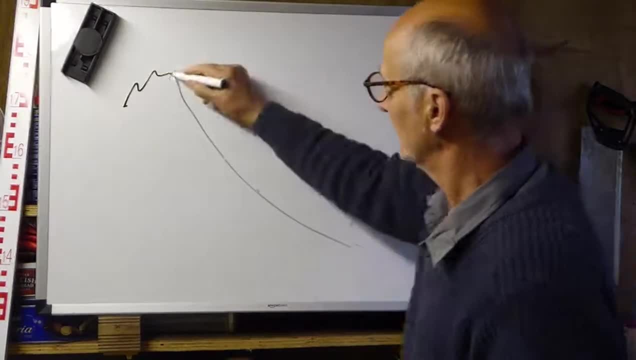 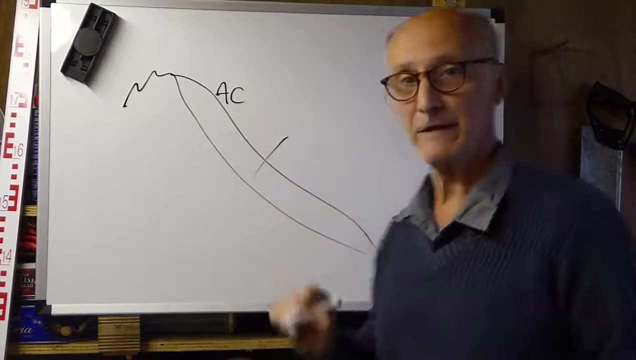 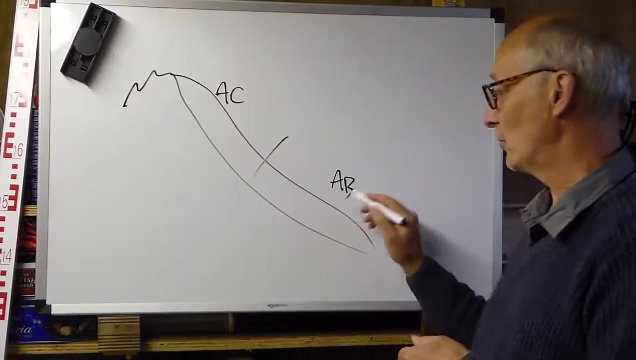 slightly different way. So you've seen the mountain glacier example, where we have an equilibrium line above which there's an accumulation area and below which there's an ablation area, with more accumulation and ablation up here and more ablation and accumulation down here, Flow of ice through the system and 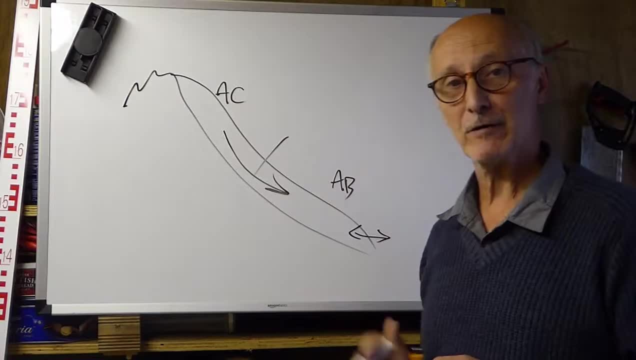 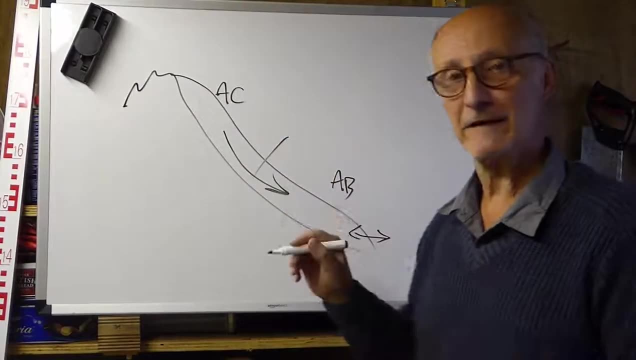 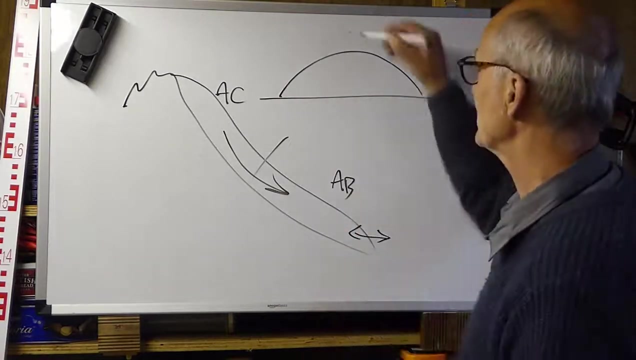 advance or retreat of the margin, partly in response to changes in mass balance through time. We drew that through a mountain glacier system and you've seen that in the in the graphics previously. You can do something very similar for an ice sheet situation where the accumulation zone is in the central area. 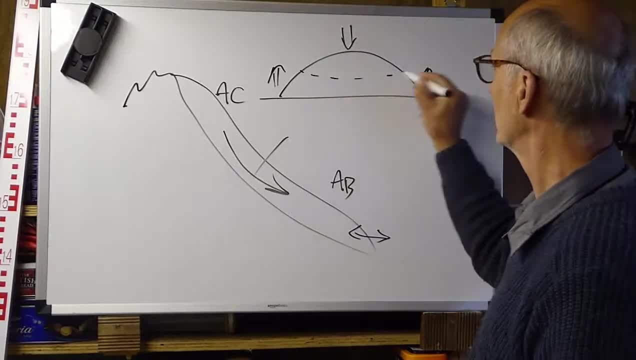 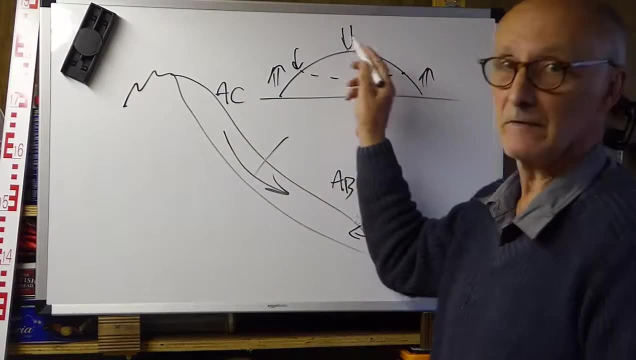 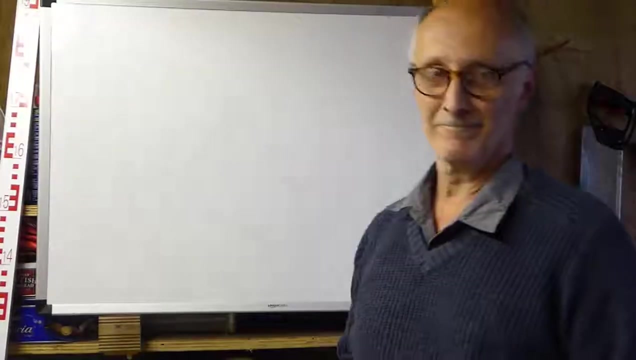 and the ablation zone is around the perimeter and the equilibrium line is altitude, runs somewhere in between the area in the middle, where there's more accumulation than ablation, and the area around the edge, where there's more ablation than accumulation. So we can also consider the mass balance through. 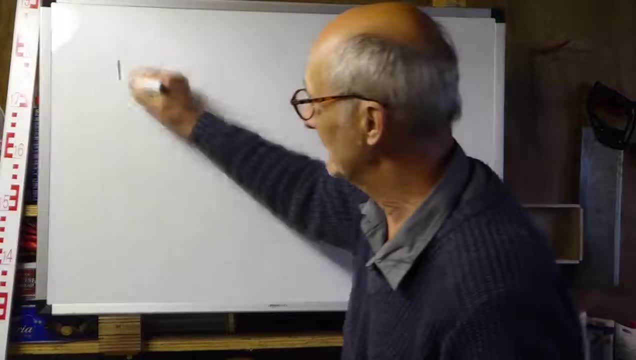 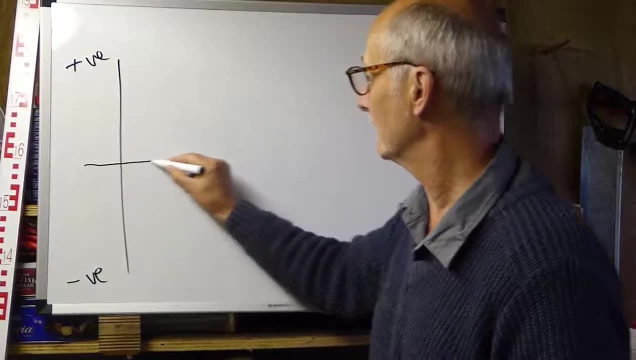 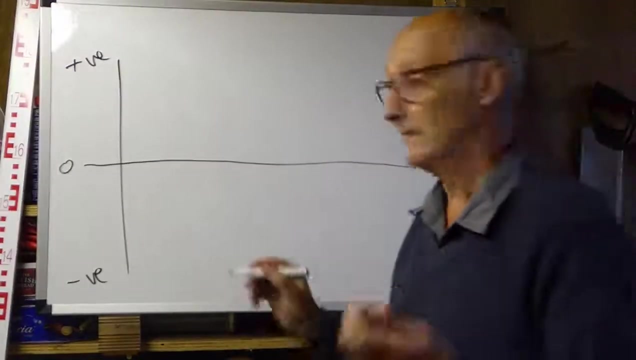 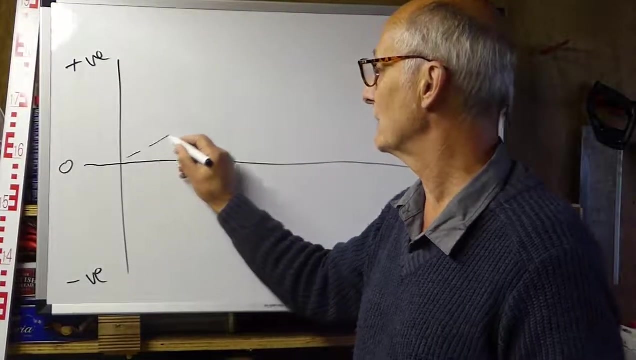 the course of a year, a mass balance year. Let's draw a graph with positive balance, negative balance, equilibrium, so zero mass balance and time over the course of a year. During the course of the winter, you would expect there to be a gradual accumulation over the course. 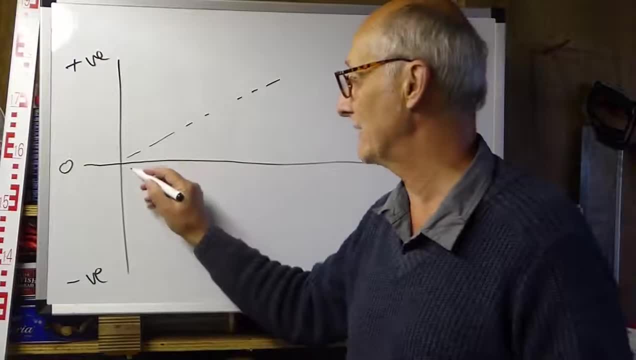 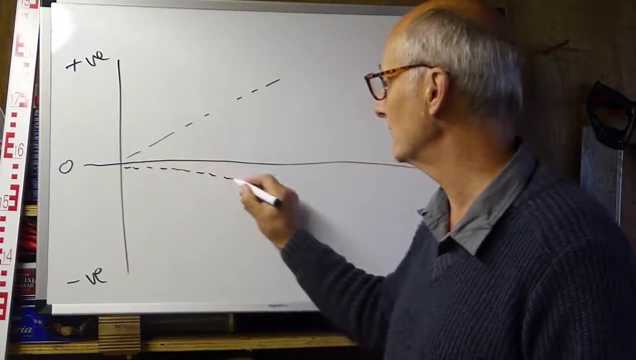 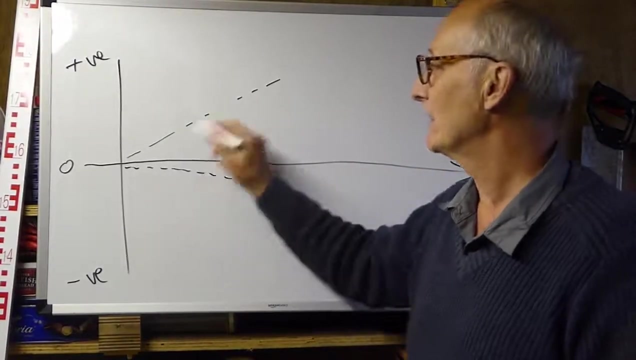 of time, There will also be some ablation during that period. so, superimposed upon that mass gain from snowfall input, There will also be some mass loss from melting carving, even during the winter in many glaciers. As we then move through into the summer, the rate of increase the positive inputs. 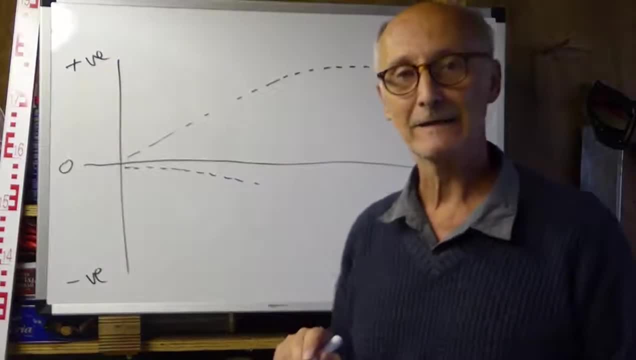 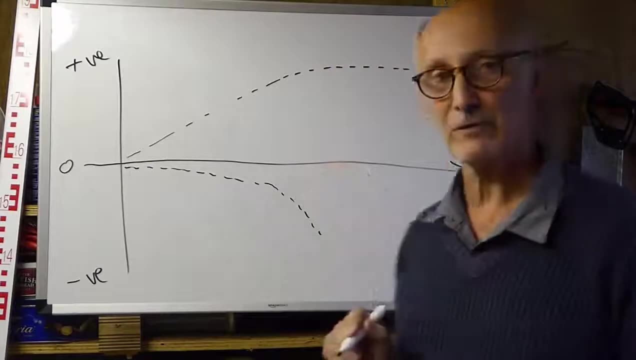 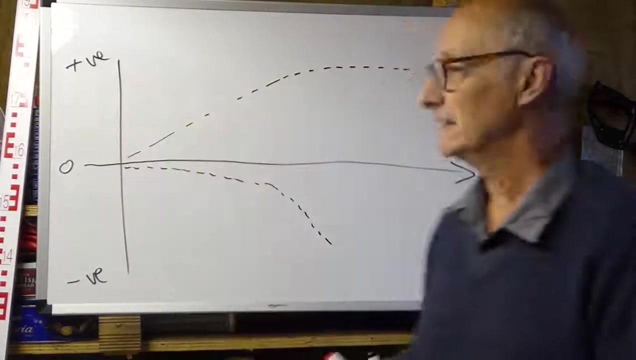 into the glacier will diminish and flatten off as we get less accumulation during the summer months and you would anticipate greater ablation. so more of a negative input during the summer, when you're losing material Over the course of the whole year. if you combine the accumulation and 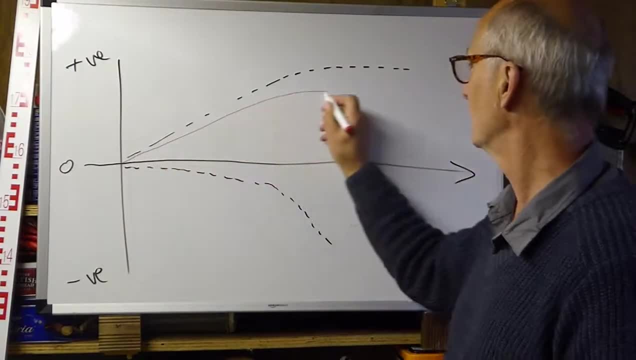 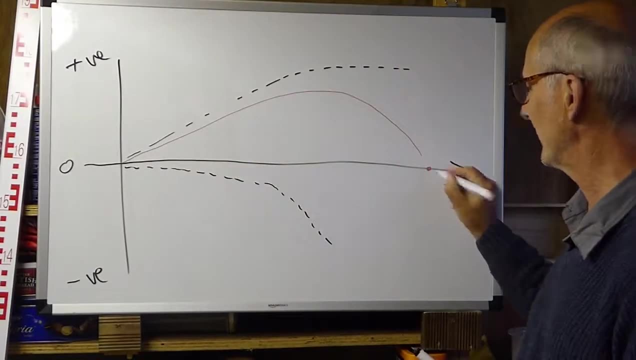 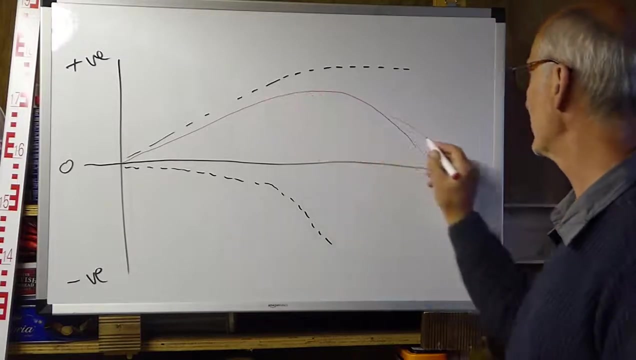 the ablation, you'll have a balance year. that looks something like that Now. if at the end of the year the line comes back to zero, then the glacier is in equilibrium, it's in balance. the balance is zero. But if it ends up somewhere above zero, then we have a positive annual mass balance, and if it 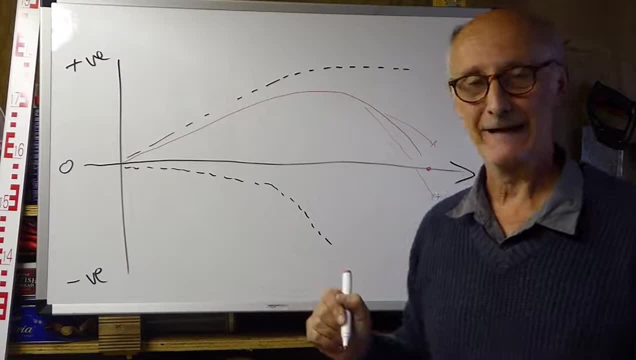 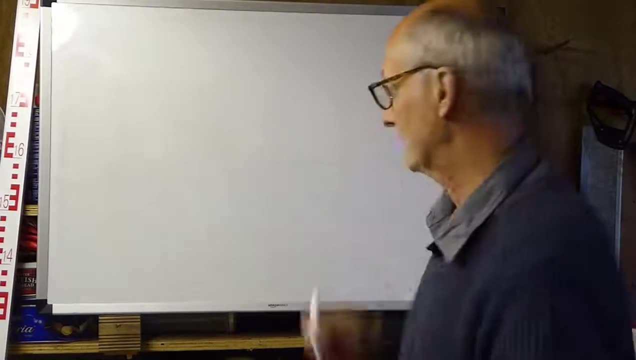 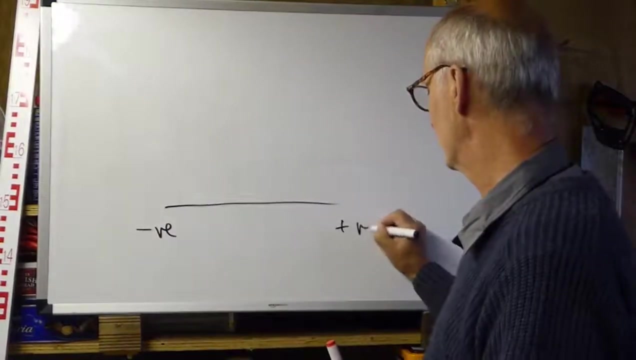 ends up somewhere below zero, then we have a negative annual mass balance. Finally, we can draw what we call a vertical net balance profile for any glacier And for that we have negative balance on the left hand side, positive balance on the right hand side. So our zero balance or our 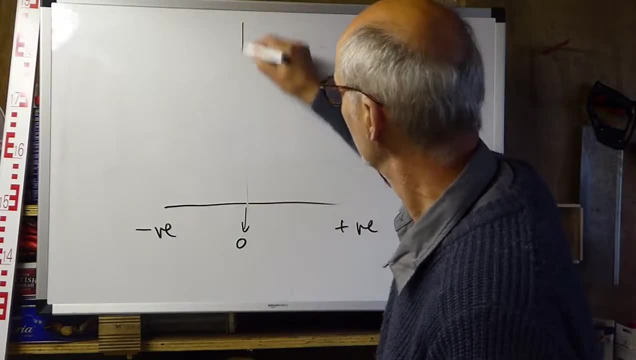 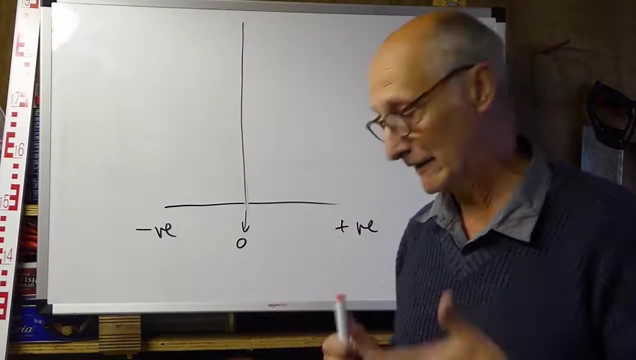 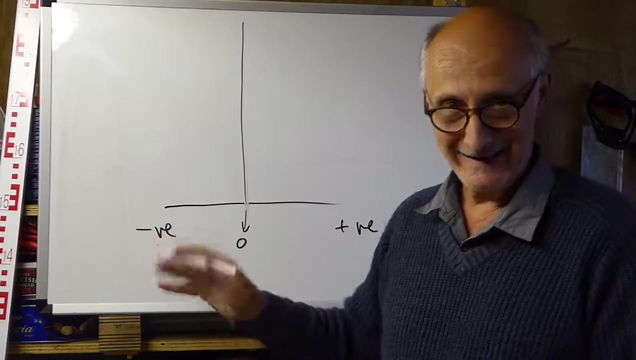 equilibrium is up the centre of the graph. So for any glacier we can draw onto here what the local mass balance is at different elevations up the glacier. So typically at the bottom end of the glacier we're going to be in a negative mass balance environment. we're in the ablation zone. 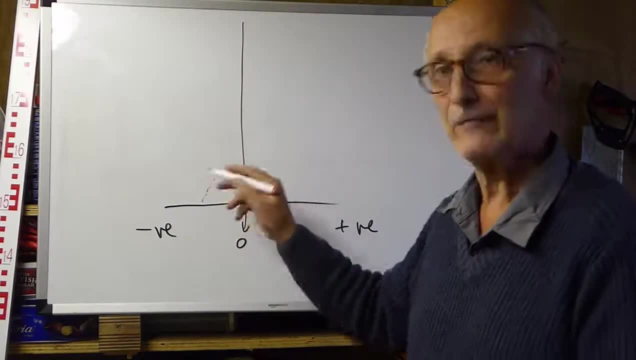 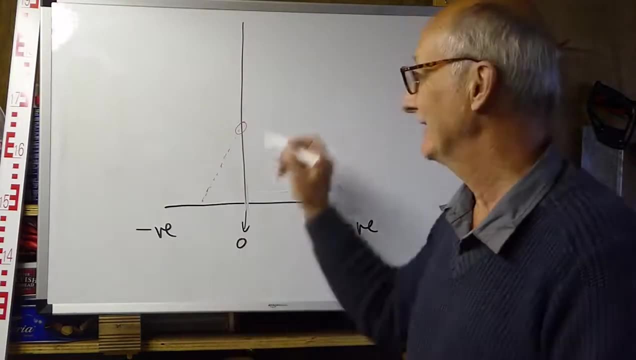 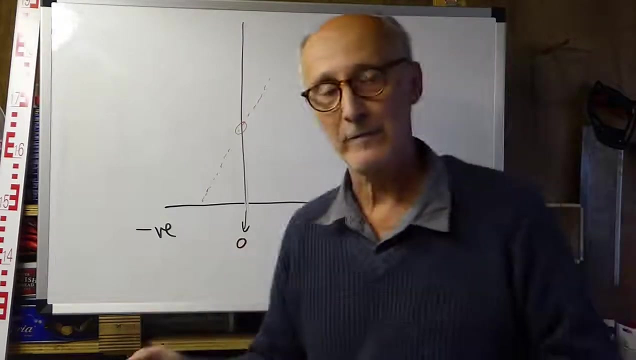 Higher and higher up the glacier, the amount of ablation is going to decrease relative to the amount of accumulation, until we reach a point where negative and positive balance out, and that's the equilibrium line for our particular glacier. Above the equilibrium line because there's more. 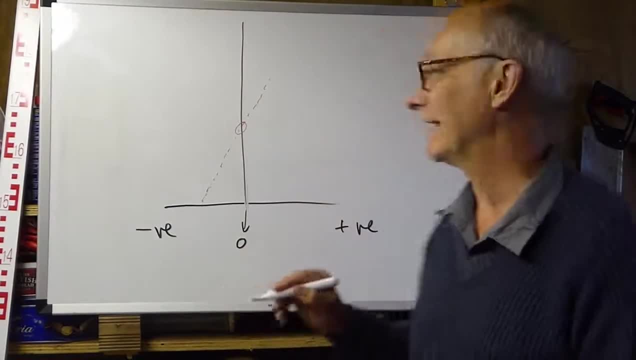 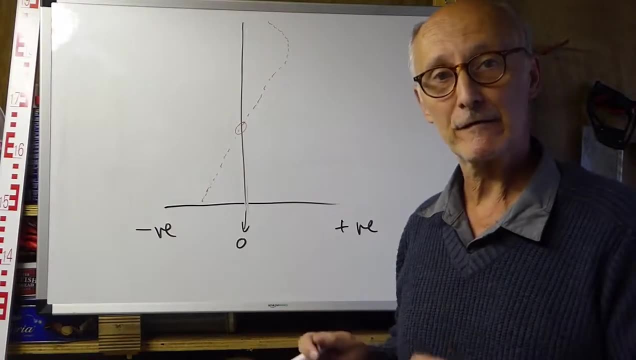 accumulation and less ablation. we're moving into a positive, balanced area. A lot of glaciers in their upper areas curve back towards the left hand side because the amount of snowfall decreases at high elevations. So in the centre of the Antarctic ice sheet, for example, there might be less. 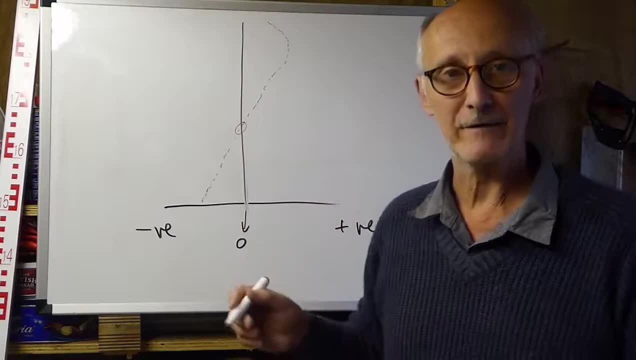 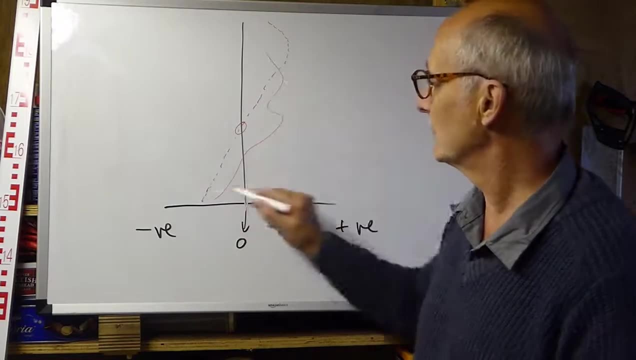 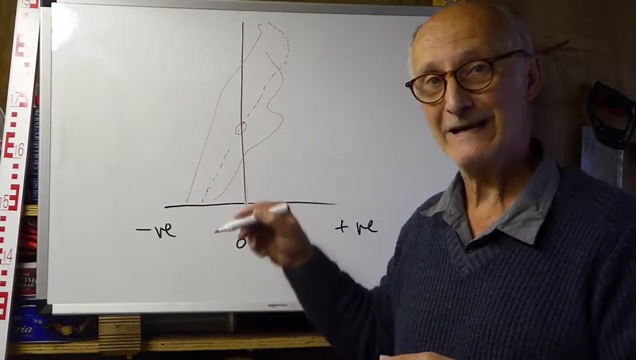 accumulation than there is closer to the edge of the ice sheet, because the atmosphere is colder and drier, not so much snow. So for different glaciers you can draw different vertical net balance profiles and you can revisit the profile for any particular glacier over the course of time and see. 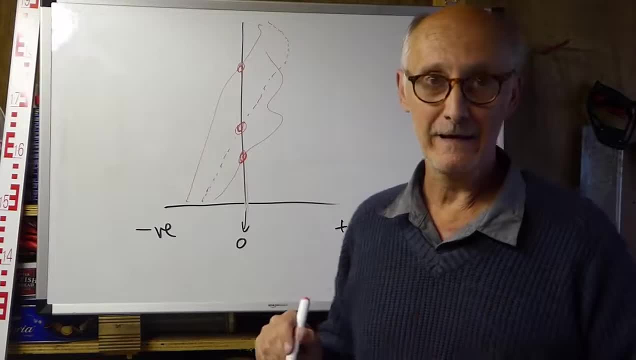 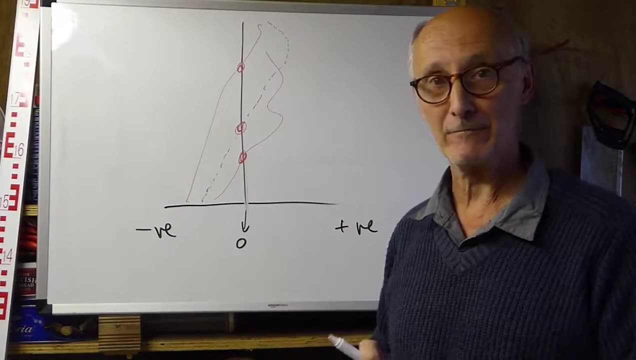 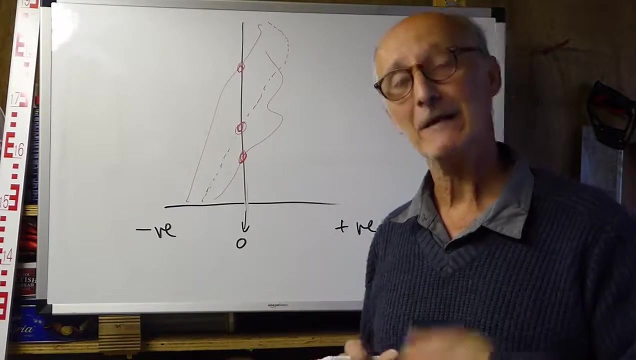 how the ELA, the equilibrium, or the equilibrium of the glacier, will change over time. So this is another interesting way to represent mass balance in a graphical form. Now I've only given you a very quick introduction to some of the ways of looking at mass balance. 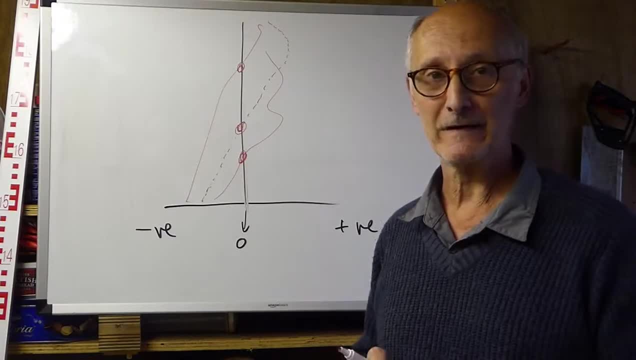 There's lots of reading for you to do on this, and I'll point you to that in other sections of this unit.